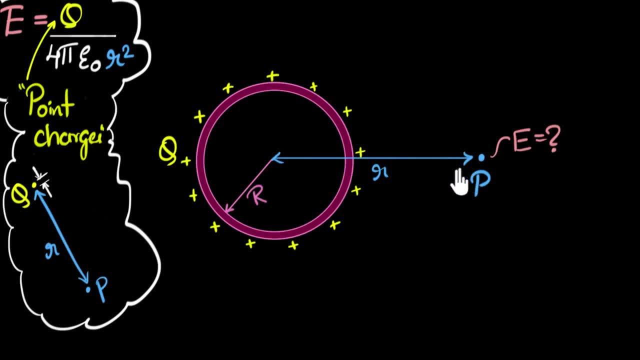 So we cannot use Coulomb's law directly. I mean think about it. What would the r over here represent? Would it be distance from this charge? Would it be distance from this charge? r is the distance from charge right Now, if the charge is distributed. 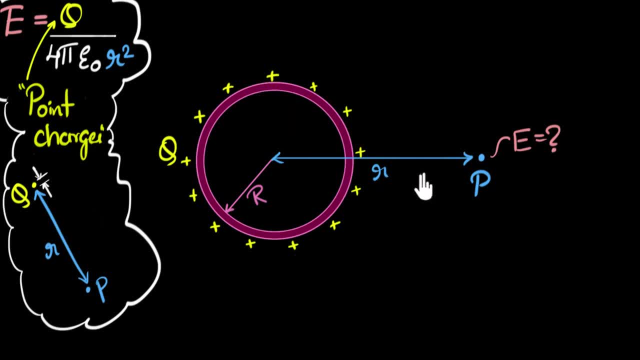 how do you figure out what r is? You can't, And so we cannot directly use Coulomb's law. So what do we do? Well, one way to solve this: using Coulomb's law. I mean, you can still solve it. 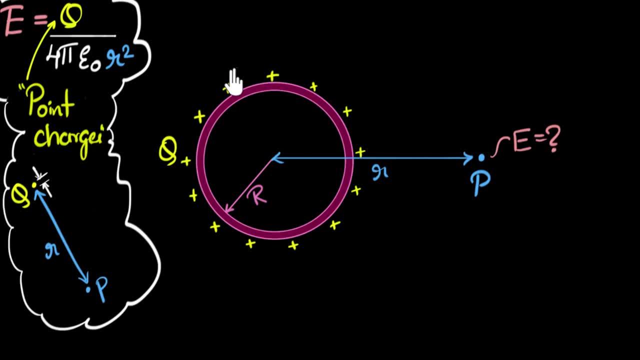 but you can't do it directly. But one way to do that is you take this charge distribution and divide it into tiny, tiny pieces. What I mean is you can first calculate the electric field over here only due to this charge, Neglect everything else. 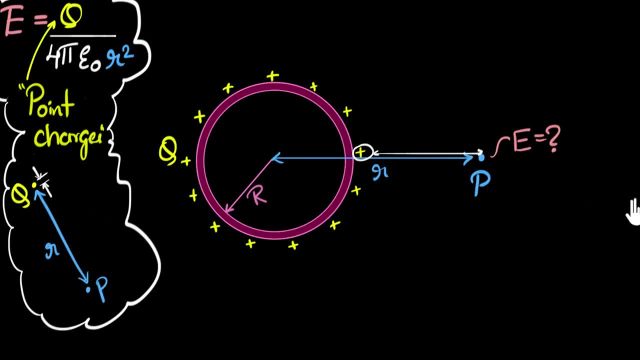 Only due to this charge calculate what the electric field is. A tiny charge over here. Then you calculate the electric field only due to this charge, Then you calculate the electric field only due to this charge, and so on and so forth, And you do that over the entire sphere. 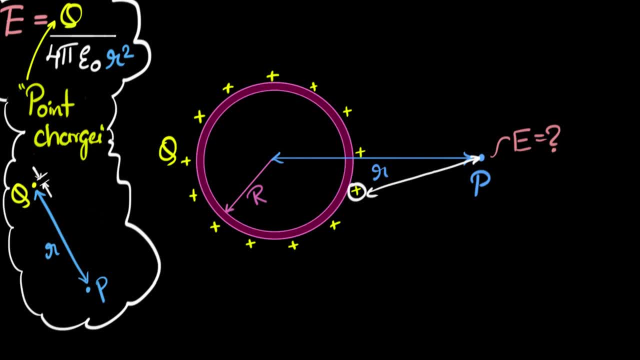 add them all up and you will get your electric field. Now does that sound tedious? Yes, it's gonna be tedious. There'll be a lot of integration involved in that, but it can be done. You can use Coulomb's law in all situations. 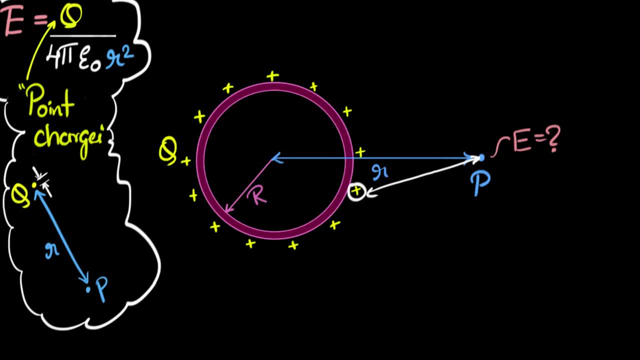 and calculate such problems. It can be done, but it's very tedious, And that's the thing about this. that's the thing I want to discuss in this video. Is there a way to solve this problem without doing complicated integrals? The answer is yes. 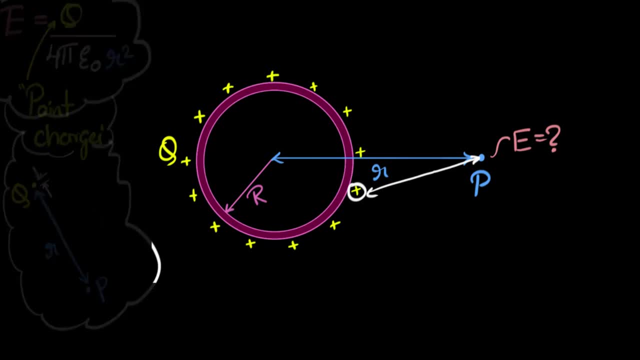 We have to. we have to get rid of Coulomb's law. Coulomb's law is not gonna be helpful for us. Let's get rid of the Coulomb's law. Yeah, Coulomb's law is not gonna be helpful, but you know what will be helpful for us? 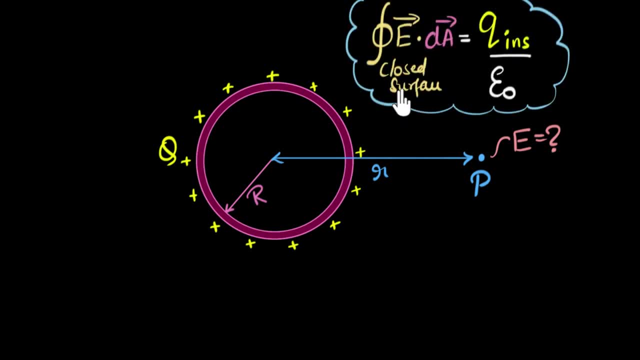 Gauss's law. Remember Gauss's law, which tells that if you take a closed surface, the flux through it will always equal total charge inside that surface divided by epsilon naught. And, of course, if you're not familiar with this, we have discussed this in great detail in a previous video. 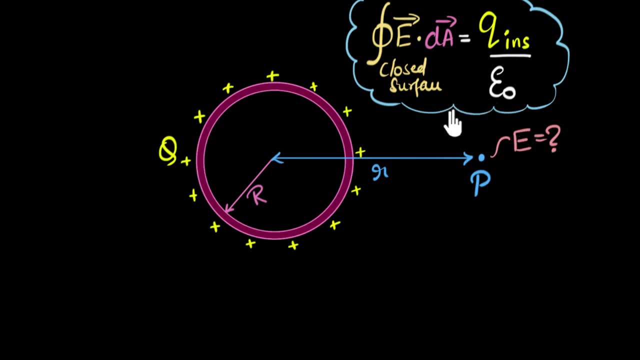 You can go back and practice as well, but we can use Gauss's law to solve it over here. Now, looking at Gauss's law, you might say: hey, how, how, how can I use Gauss's law Even there? also, there is an integral right. 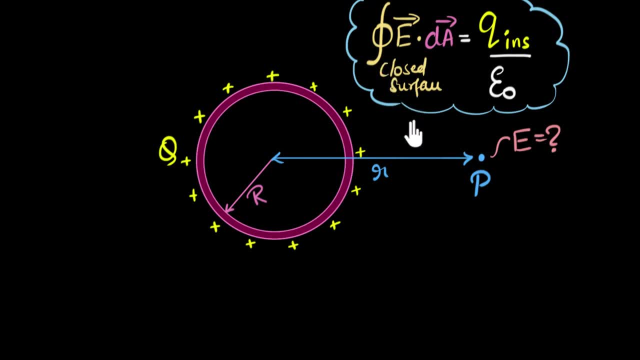 Isn't this also gonna be complicated? The whole point of using Gauss's law- and this will be true in any problem that we use Gauss's law- The whole point is you choose a closed surface such that the electric field everywhere on that surface. 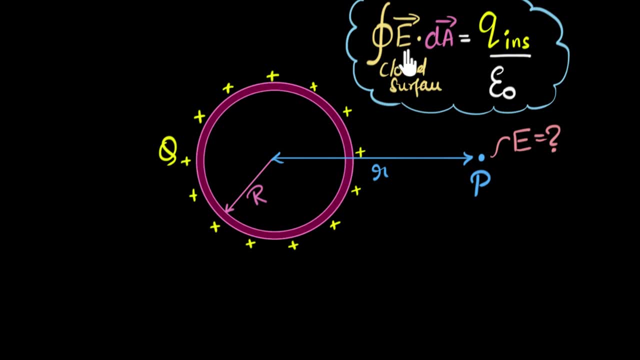 is gonna be the same- at least in most cases it's gonna be the same- then that electric field can be pulled out of this integral, as you will see, and then the mathematics becomes very simple. you don't even actually have to integrate. 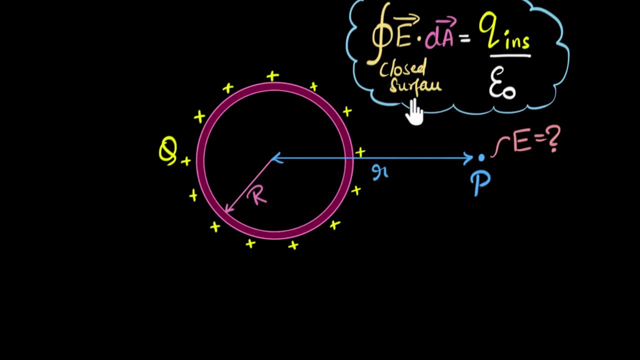 That's the whole idea. So you can't do this for all cases, only in certain special cases, in permanents, which is called the freeori. so that's the idea. Okay, so for this extra matrix I am not gonna be using Gauss's law. 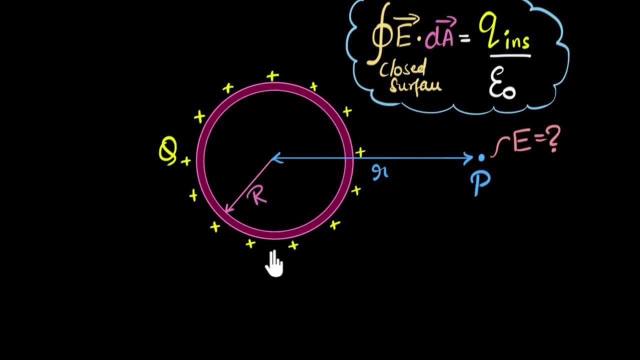 cases you can choose such a closed surface, and we will see. this is one of those special cases, and so the whole idea is: in such special cases, let's not use coulomb's law, let's use gauss's law to solve the electric field. okay, so let's begin. i'm pretty sure you're excited, so the first step would be to 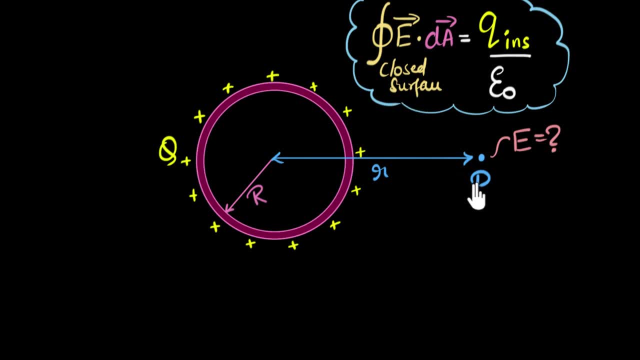 choose a closed surface right? what kind of closed surface would i choose over here? before answering that question, we need to first look at what the electric field looks like everywhere. only then we can choose an appropriate closed surface. so let me get rid of this equation for a while. 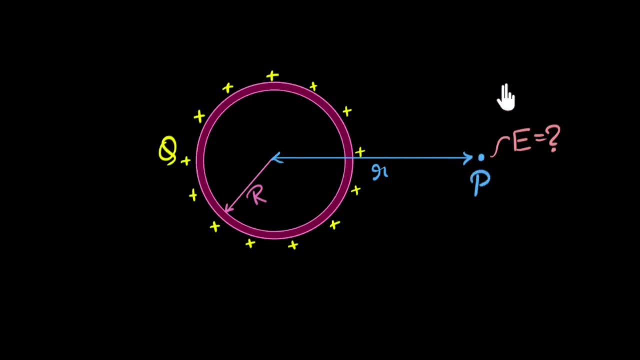 and think a little bit about what would the electric field look like everywhere outside. inside we'll come back a little bit later- but think about outside, given that it's a spherical distribution, it's a spherically symmetric meaning. you know the charges are uniformly distributed. because of that, we will find that the electric field everywhere has to be along the radius. 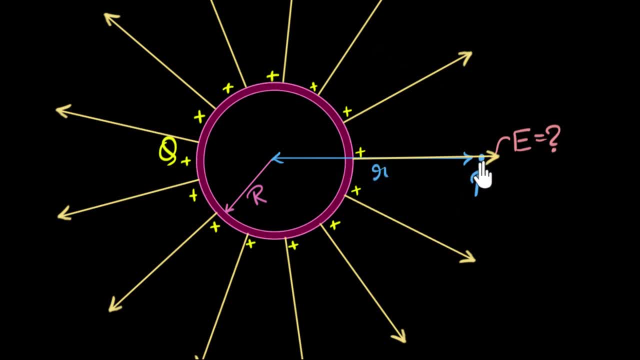 it's going to be a radial field and we will find that the field at a distance r at any point. if you go any point at a distance r, you will get the field value to be exactly the same. so radial field whose value only depends upon the distance from the center. but of course, the question could come into your mind: how do i? 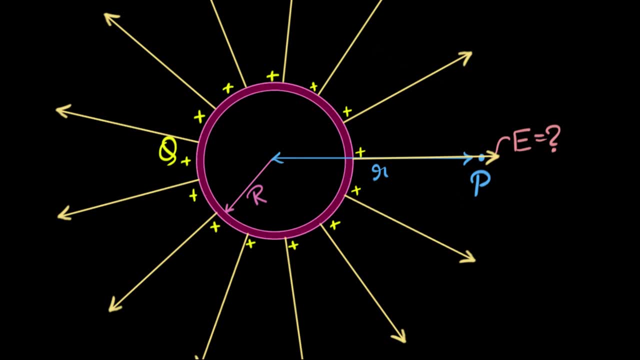 know this. how, why should it be radial? and that's really important. i want to ask a lot of why? questions over here, because a lot of details involved. so conceptually, this is very, very enriching. so if you had to convince this to someone, how would you convince them? why would the field be? 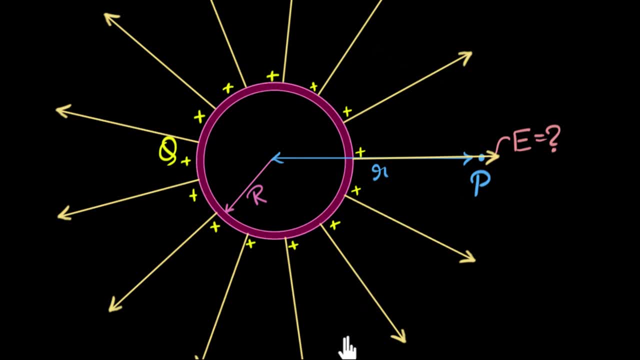 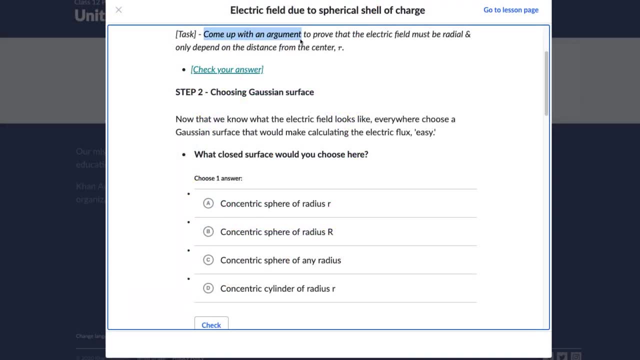 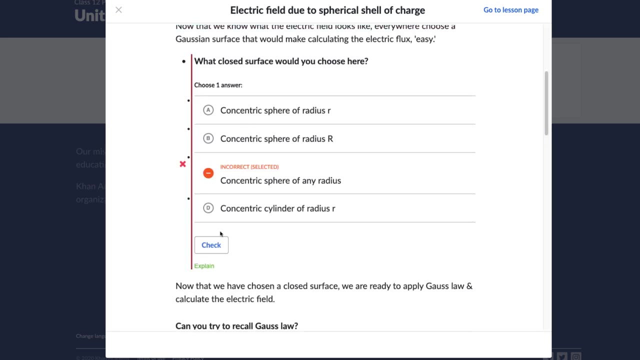 radial. in fact. guess what i want you to explore and interact with this derivation. so let's continue this in our article on our website, where you get to pause and wonder if you're stuck. you can always get the solution. you get to try each step yourself. it will be kind of rediscovering the whole. 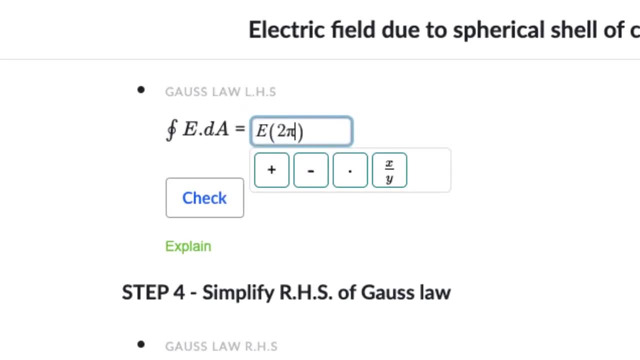 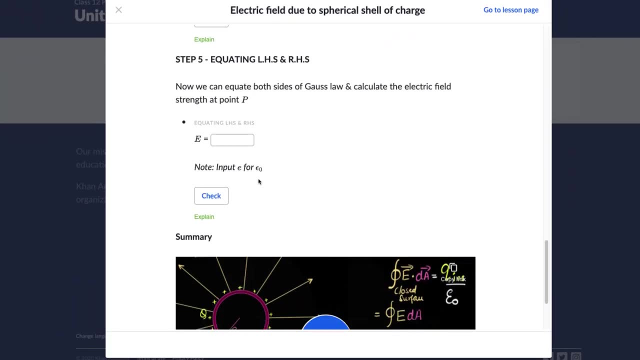 derivation yourself, so it won't be just me talking and telling you what to do, like in a normal video. yes, of course this will take a little longer, but i believe your learning would be more solid and fun. and, of course, if you're watching this on youtube, then here's a link to continue on to our free 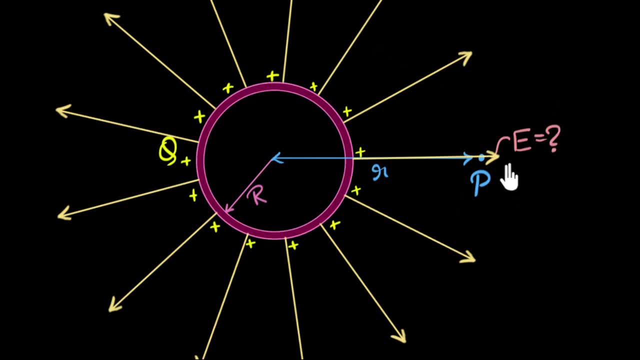 website. so the next step would be for you to come up with an argument as to why this field is radial, should be radial. 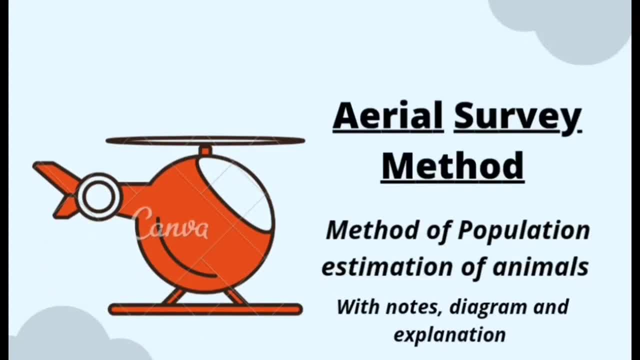 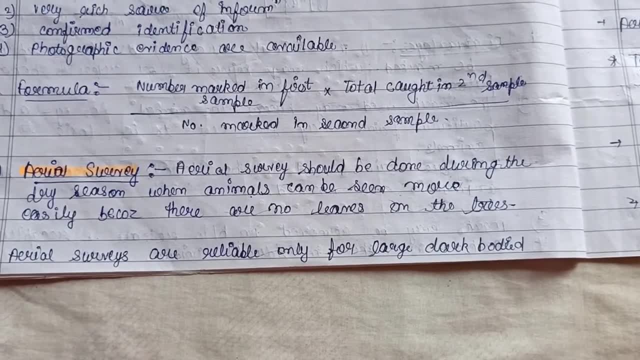 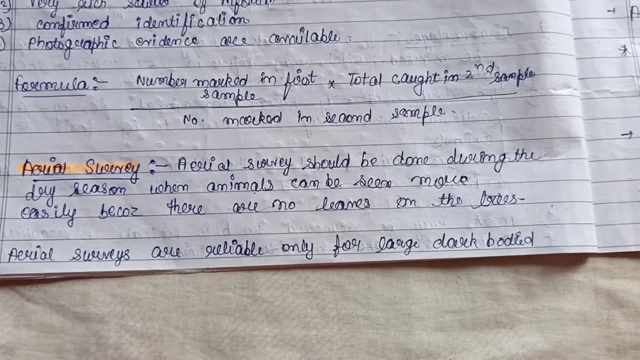 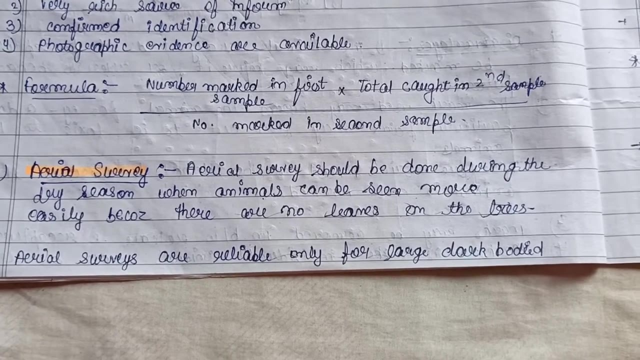 Hello everyone, welcome back to my channel. so earlier we have discussed about the methods of the population estimation of animal and we have discussed about the census method, the quadrate method and the mark recapture method. today we are going to study about the aerial survey method and the sampling method. so aerial, 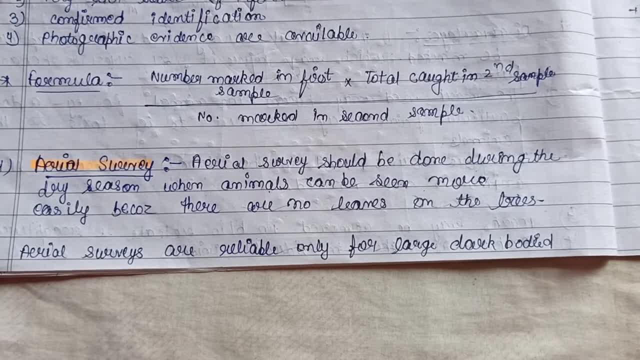 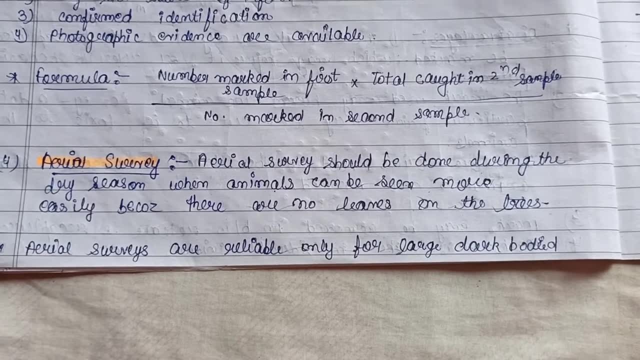 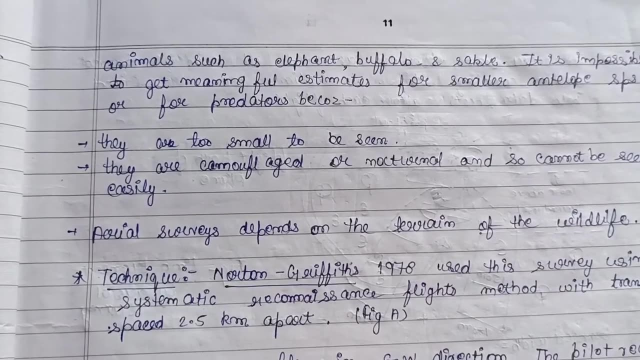 survey should be done during the dry season only. that is when animals can be seen more easily because there are no leaves on the trees. so aerial surveys are reliable only for large and dark bodied animals such as elephant, buffalo and the savon, so it is impossible to get them. meaningful estimates for the. 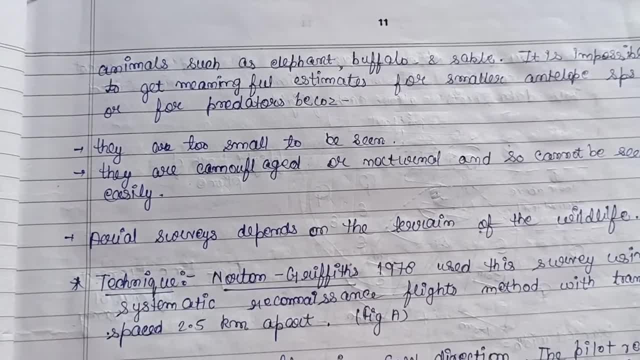 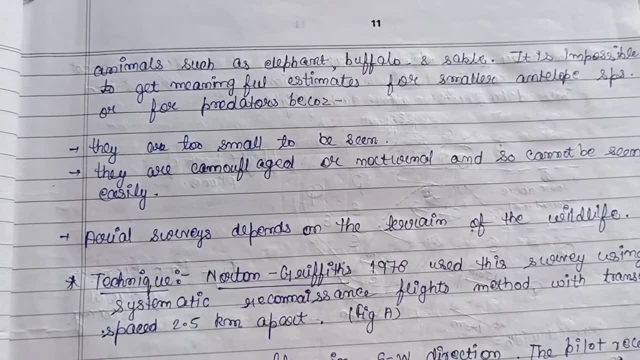 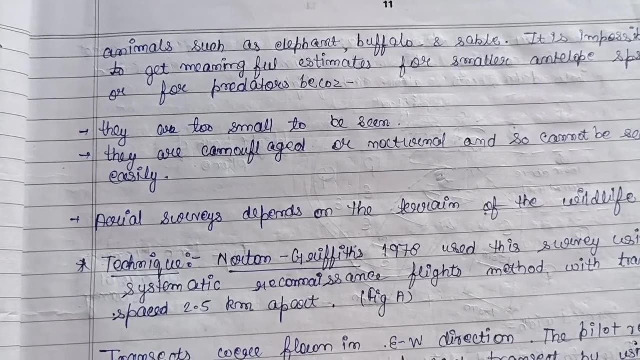 smaller antelope species or for the predator species, because they are too small mold that is to be seen and they are camouflaged or nocturnal so they cannot be seen easily. the first thing is their size is very small and another is they basically came out in the night. 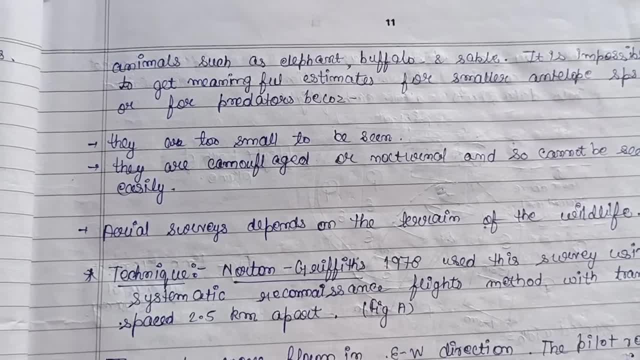 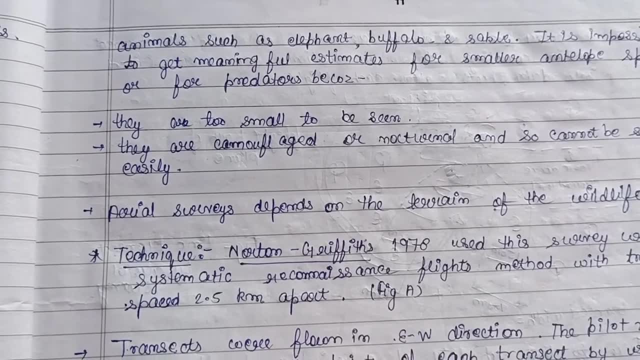 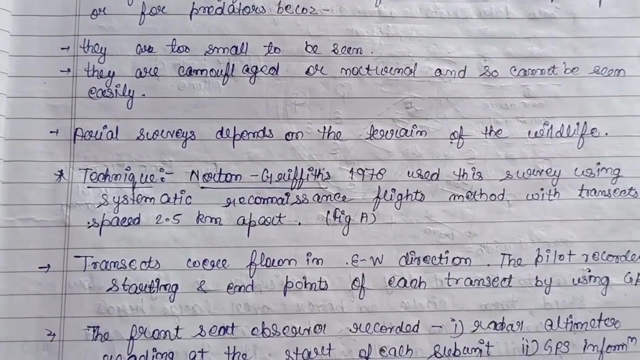 only and perform all their activities in the night, that is, they are nocturnal, and if they came out in the day, they camouflage themselves, that is, they change their color or size according to the surrounding environment, so they are not easily seen. according to the aerial survey. aerial surveys. 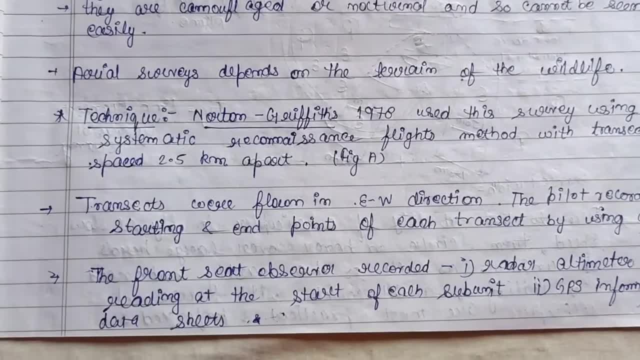 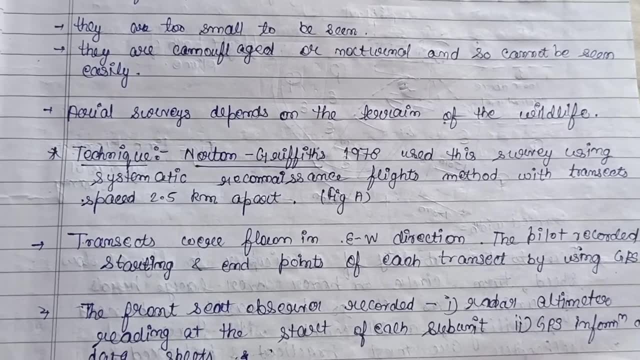 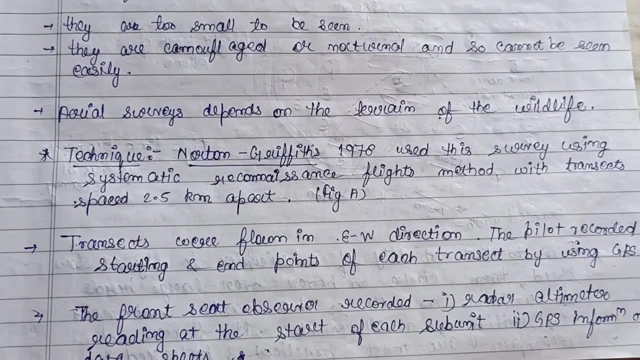 depends on the terrain, of the wildlife. so there are techniques for the aerial survey. Norton Griffiths in 1978 used this survey using the systematic reconnaissance flights method with transects spaced 2.5 kilometer apart. so transects were flown in east-west direction. the pilot recorded: